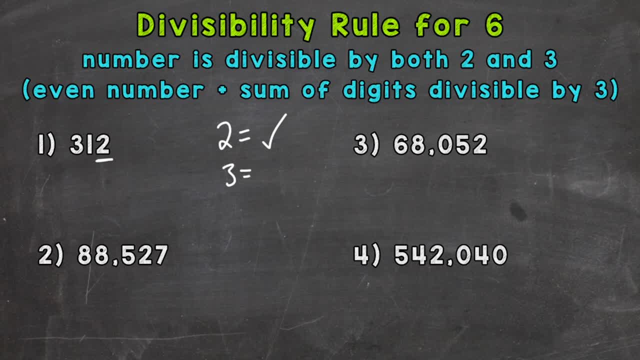 then the original number is divisible by 3.. So we'll add 3 plus 1 plus 2.. 3 plus 1 is 4, plus 2 is 6.. So is 6 divisible by 3? Can we do 6 divided by 3 and get an answer without a remainder? 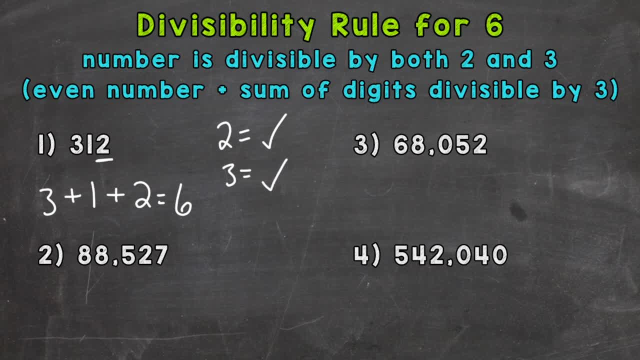 We get 2.. So, yes, 6 is divisible by 3,. the sum of the digits, Therefore the original number 312, is divisible by 3.. Since that number is divisible by both 2 and 3,, it is divisible by 6.. 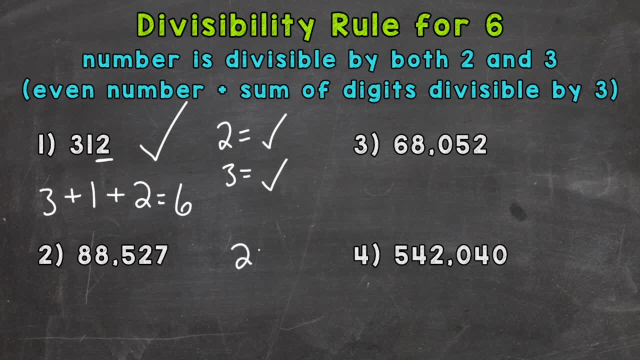 On to number 2.. So let's see if this is divisible by 2.. This number ends in a 7.. 88,527 ends in a 7.. So it's an odd number, Therefore not divisible by 2.. 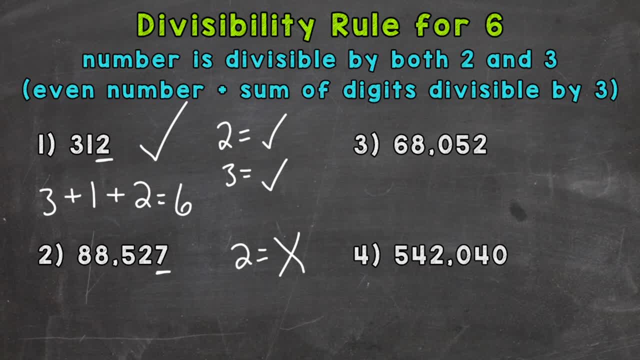 Since it's not divisible by 2, we automatically know that this isn't divisible by 6, because, remember, it needs to be divisible by both 2 and 3.. So there's no sense in trying 3 there, because we know that it's not divisible by 6,. 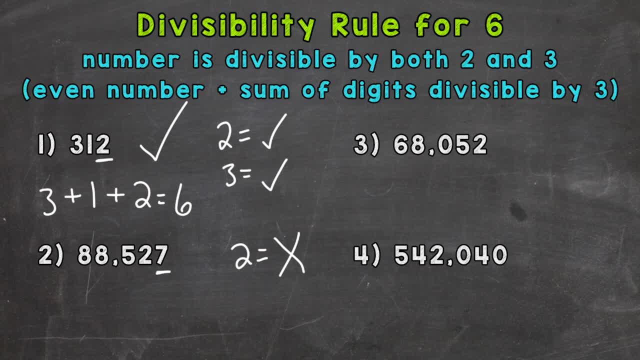 based on it being not an even number. So on to number 3, we have 68,052.. This number ends in a 7.. It ends in a 2.. It's an even number, so it is divisible by 2.. 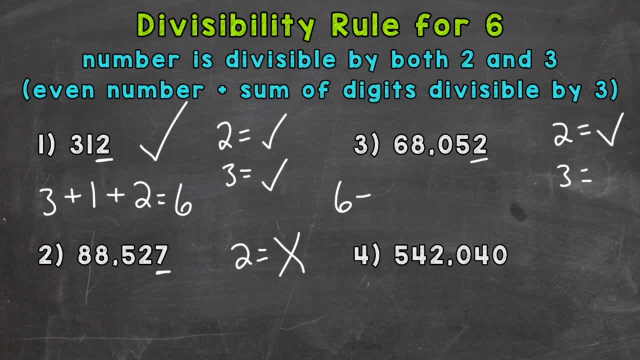 So let's try 3.. 6 plus 8 plus 5 plus 2.. Remember we need the sum of the digits. 6 plus 8 is 14, plus 5 is 19,, plus 2 is 21.. 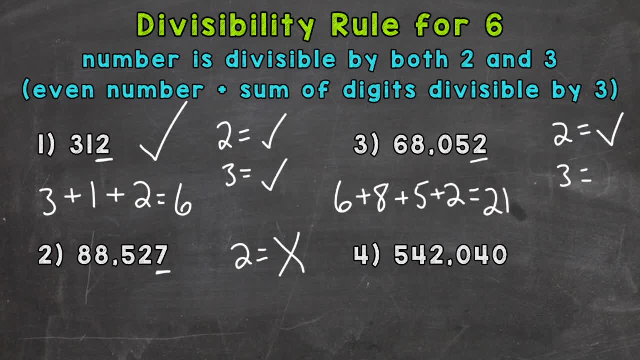 So is 21 divisible by 3?. 21 divided by 3 is 7, without a remainder, so it is divisible by 3.. 68,052 is divisible by both 2 and 3.. Therefore divisible by 6.. 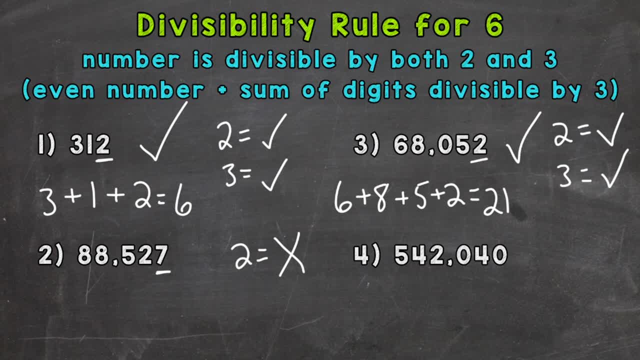 So let's move on to number 4 here, where we have 542,040.. So let's check to see if it's even. And yes, it ends in a 0, so it's an even number. It's divisible by 2..